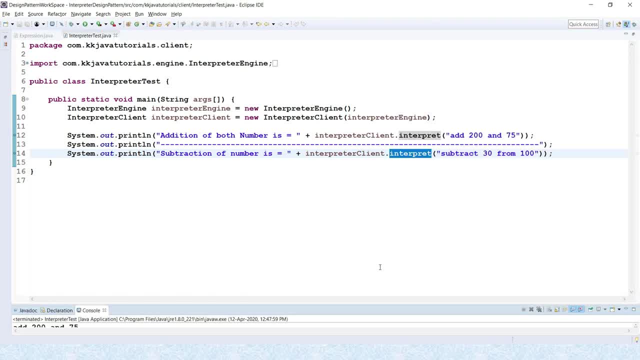 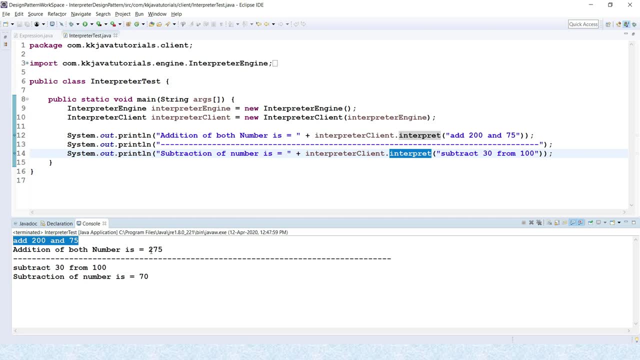 here it says: for first input, first input, this is the input right. add 275, so saying that addition of both number is 275. similarly, subtract 30 from 100, so this is saying subtraction of number is 70, so 100 minus 30 and it's comes 70. 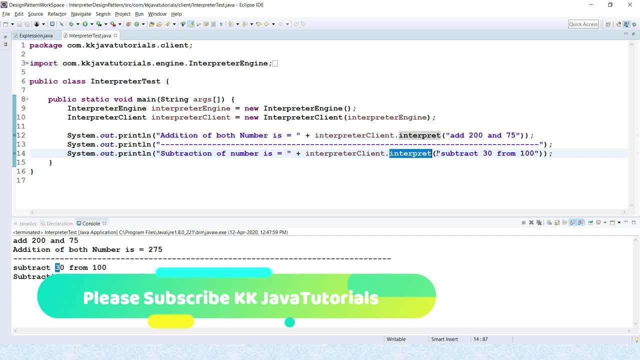 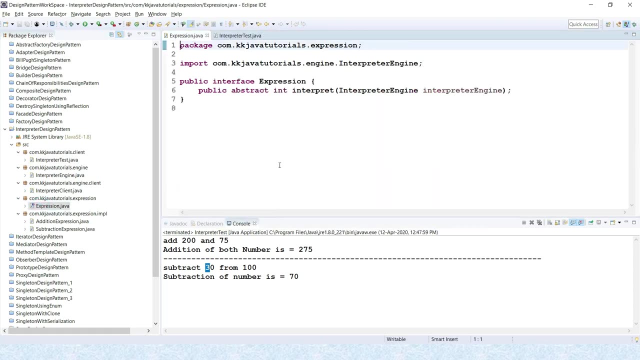 right. so here just, we are calling interpret method by passing one sentence, and interpret is able to identify whether has to do addition or subtraction. so let's see how we have achieved this one using interpreter design pattern. yeah, so first of all we have an expression which is having a 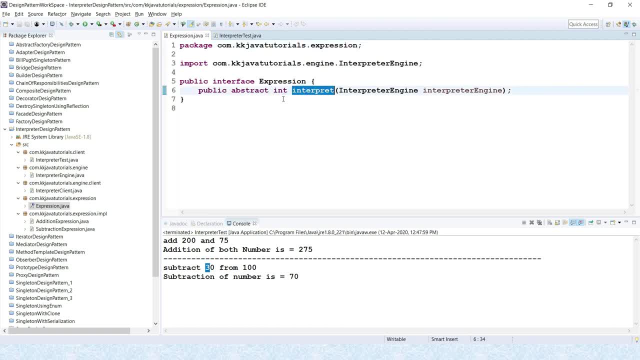 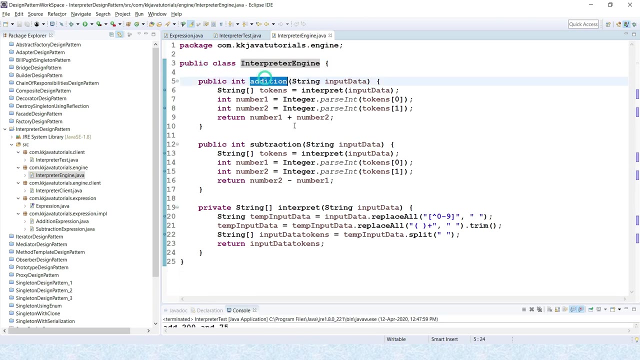 method is called interpret. return type is integer, because we want to perform addition or subtraction and this guy is accepting a reference of interpreter engine. so this is a concrete class. if you look in this class, this class is basically taking performing some action like addition and subtraction, and this is 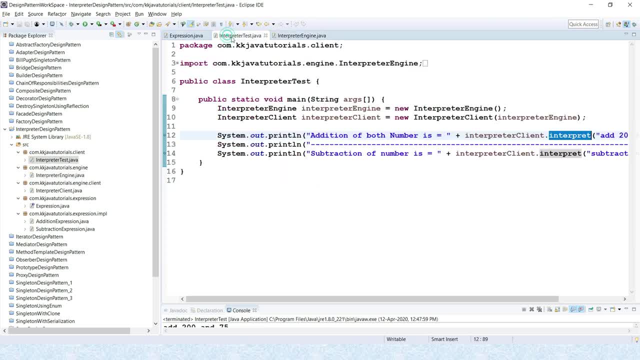 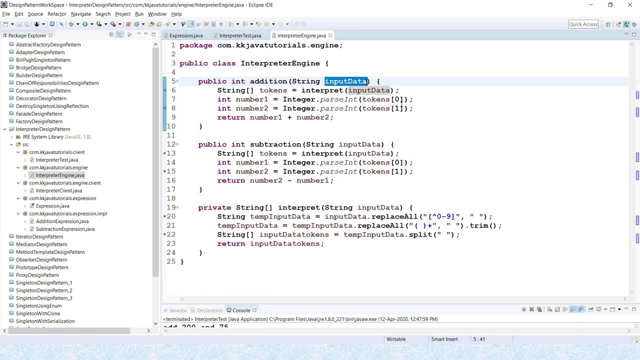 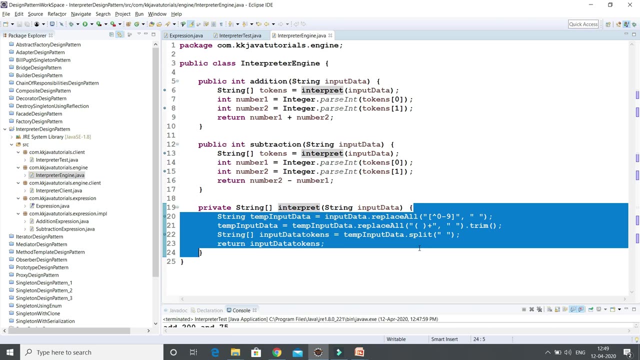 basically accepting user input. so your input is nothing but the. what input we are sending over here, right, this input that is going to send to this interpreter engine, interpretive engine basically calling this interpret method. interpret method, basically, that's making use of the regular expression and that is. 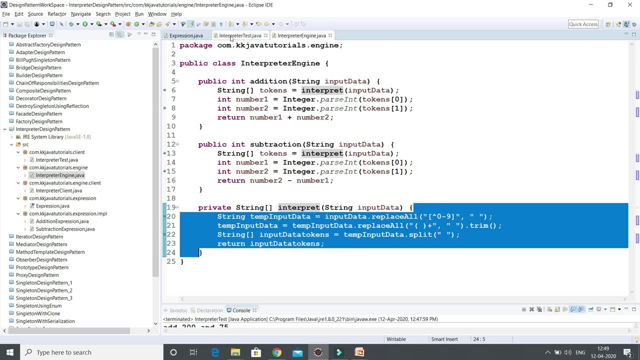 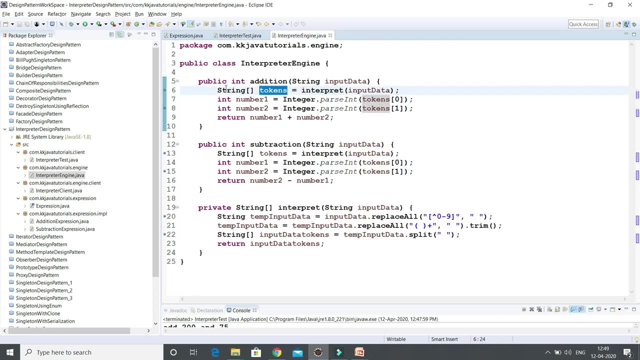 extracting all the numbers out of this input number, what we are sending over here, right, and that it does as a token- token of a string or a string array. now we are just taking both number out of this tokens array and performing addition or subtraction based on the 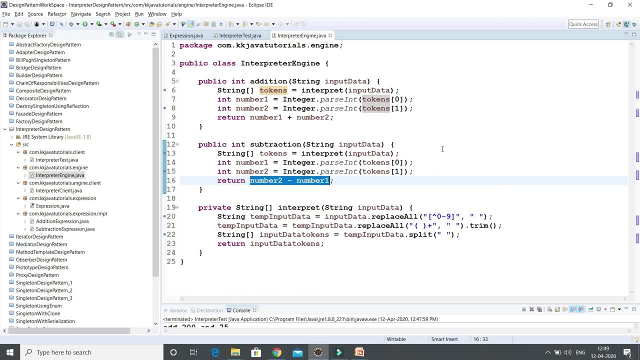 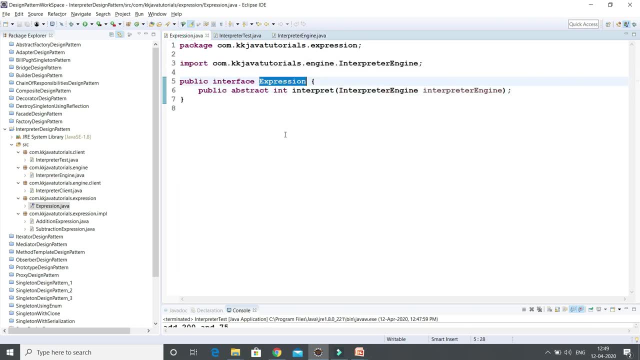 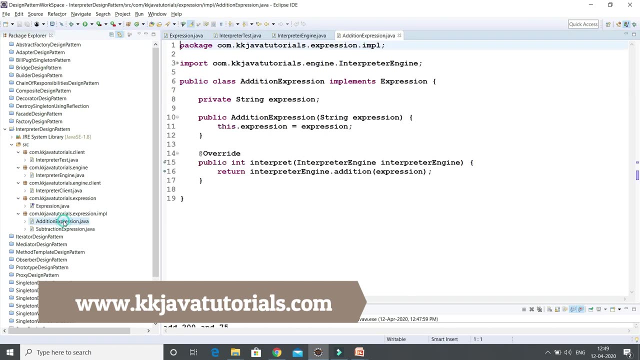 basically user desired operation, right? so now let's come to this here. so we have an expression, we need to have an expression, we need to have an expression, we need couple of implementation of this guy, right? so that's what we have: addition, expression and subtraction of expression. so addition, expression, this 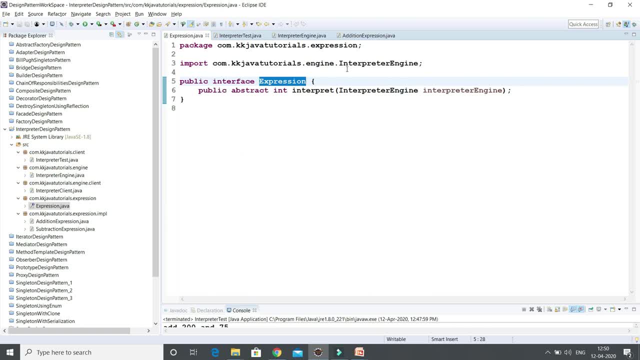 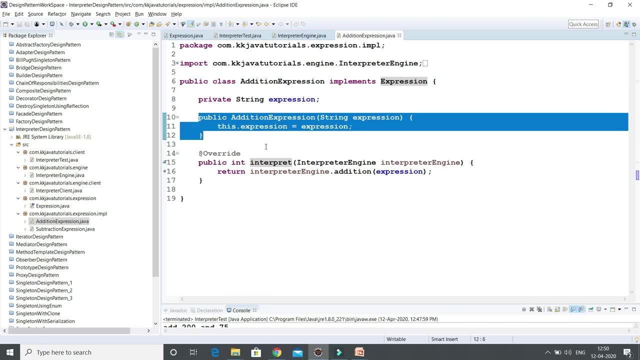 implements this expression interface here and basically this provides expression as an input right to this constructor and we have to override interpret method of this interface, right? so that's what we have over it. now. interpreter is that is going to call addition? right, this is having an edition method and similarly we have 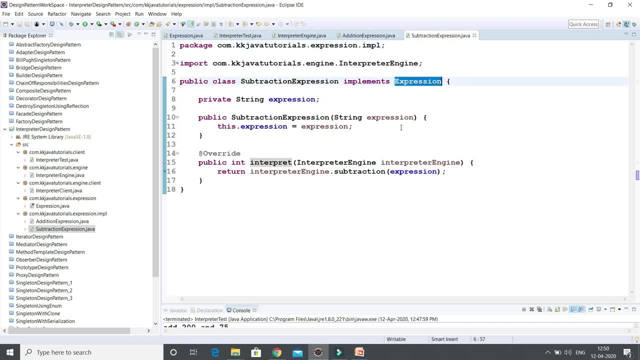 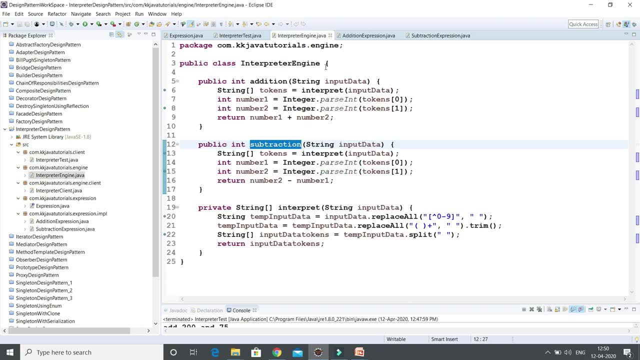 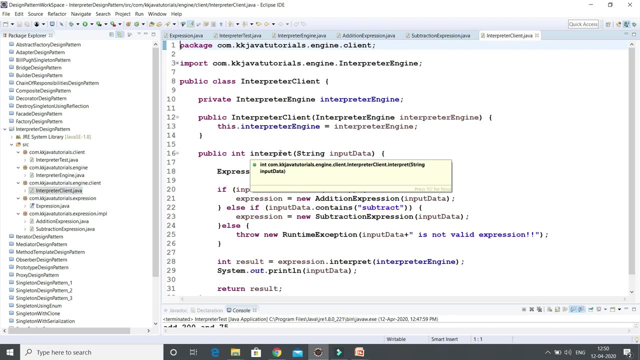 implemented subtraction expression, which also implements expression and that schools does subtract method of basically interpret interpretive engine. right now we have our last button on the least. we have a interpreter client that is going to use by the client. all right, so here this interpreter of client, basically using our reference of 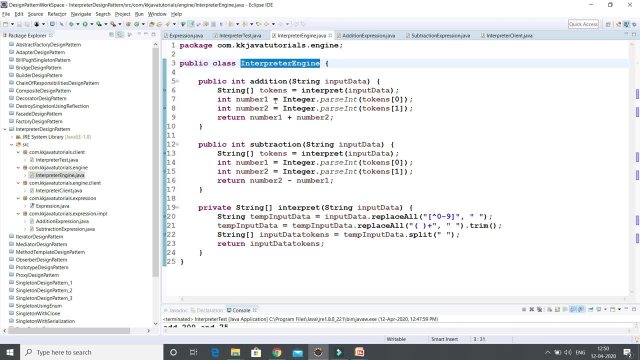 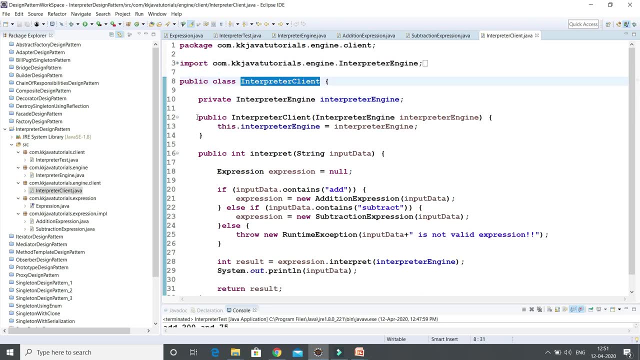 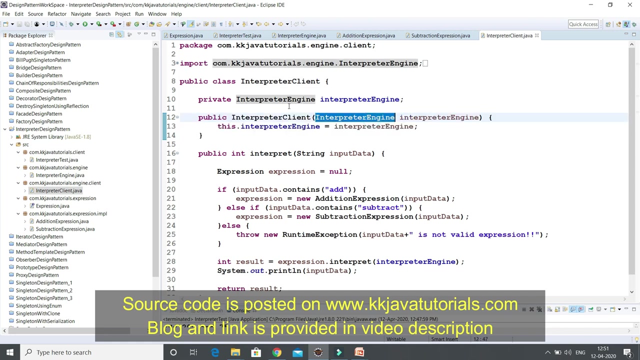 interpreter engine which is having addition and subtraction action method. now this actually actually constructor of this class is accepting a reference of interpreter engine. so if client wants to use interpreter client, then client has to basically create an object of this class and before that client has to create an object of interpreter engine that has to pass to this. 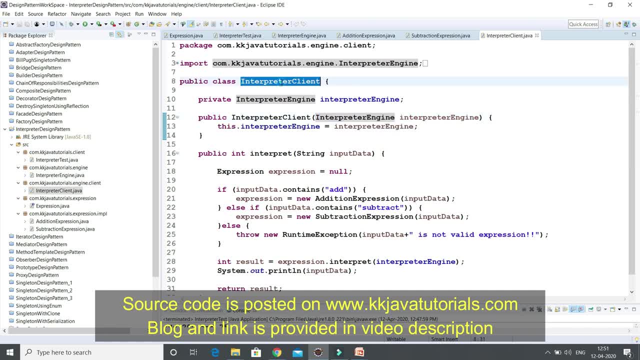 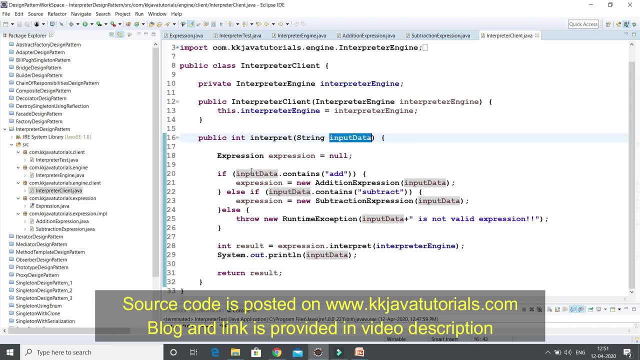 constructor right. once client is having an object of this class, then client can call this interpret method by passing its input, their input right. so now here we are going to check. if input contains literal is called add, right, then we are creating an object of addition expression by passing input. 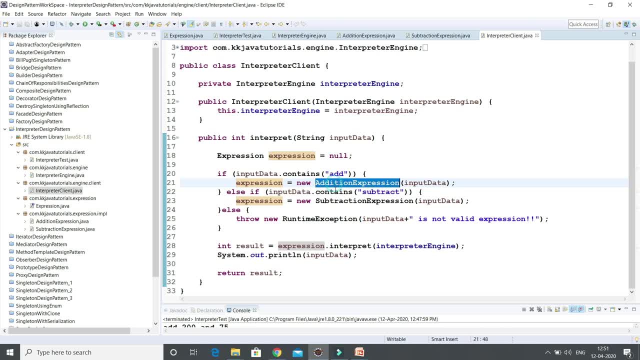 and assigning to this expression. because this, these two class- addition expression and subtraction expression- implements this expression interface right. if input, input data is contained literal, is called subtract, then we are creating an object of subtraction expression by passing input and assigning to this, basically, expression reference. now, if input data doesn't contain add or subtract, 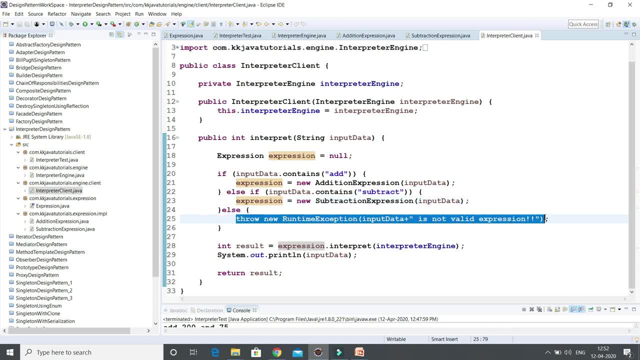 listing literal, then just we are throwing an exception. here you have opportunity to create a any kind of some exception, and then you can throw and caller can. basically you can propagate exception. you can propagate exception from here and caller has to handle. but here just I have done a runtime. 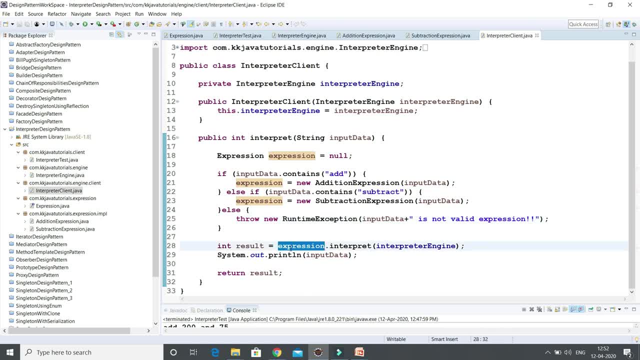 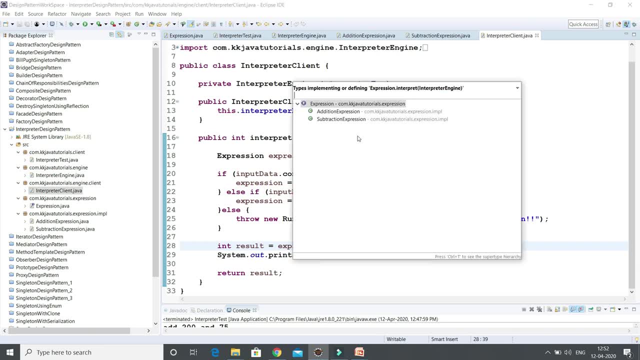 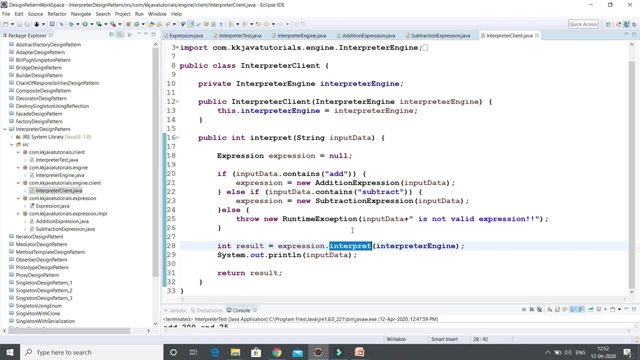 exception. that's it now. now we have an object of expression, now we are calling interpreter method. so this method is available in both the classes- right- addition expression and subtraction expression. so which class interpreter method will be called that? it's going to be called an interpreter method if that reference is stored in this reference. if, if this 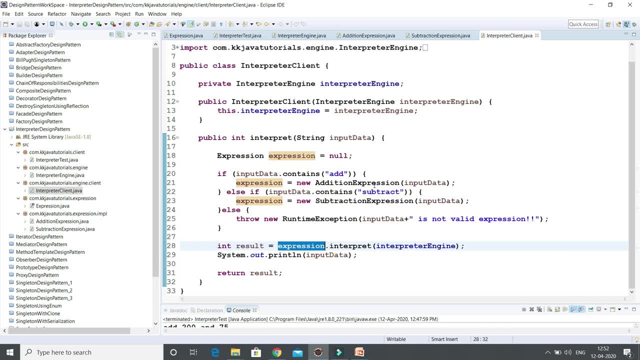 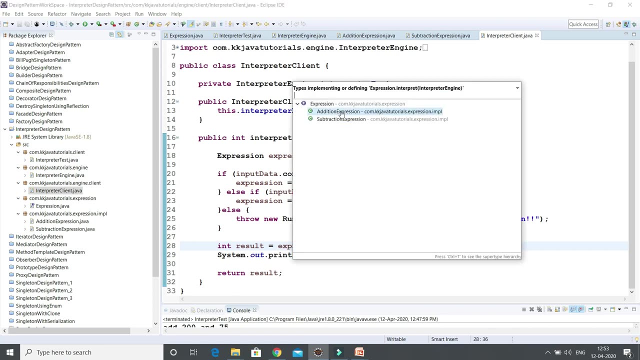 reference stores an object of addition expression, then interpret method of addition expression will be called. else, if, if that that reference store an object of subtraction expression, then subtraction expression interpret method will be called. yeah, so if you look into this, these two classes is having this, uh, interpret method here. 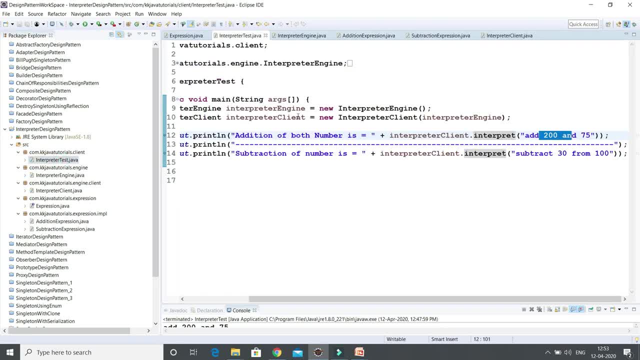 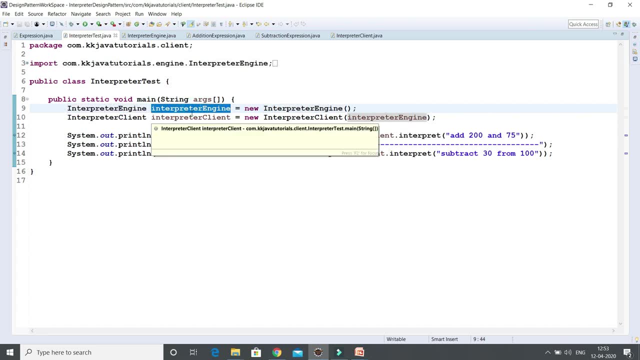 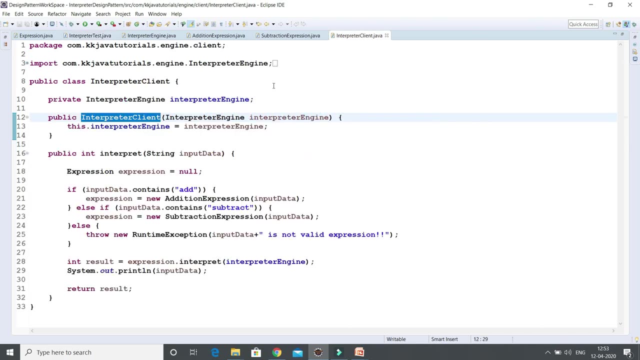 now let's run this application already. i ran this application. so here, if you look into the client application, so first of all i have created an object of interpreter engine and then i'm trying to create an object of interpreter client which demands me to pass interpreter engine object right. 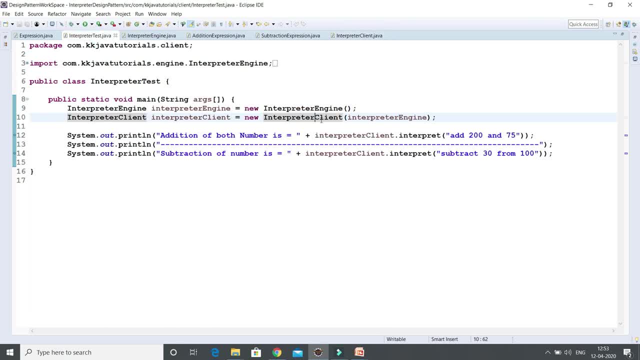 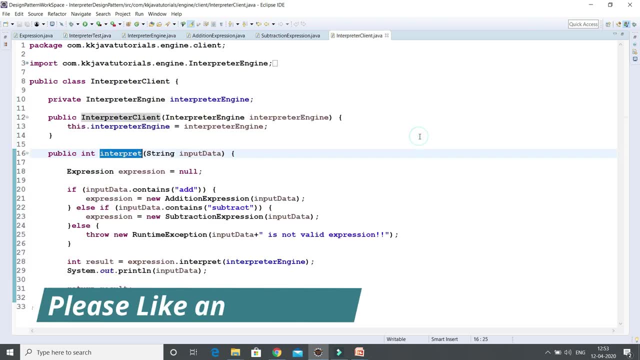 so that's what we have passed: interpreter engine object right here. now we got the an object of interpreter client. now we are calling interpret method of this uh uh, this class right now, if we pass, now we are passing the basically uh input data right to this interpret and based on the. 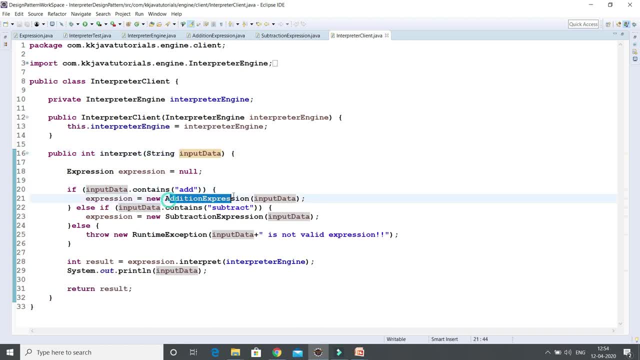 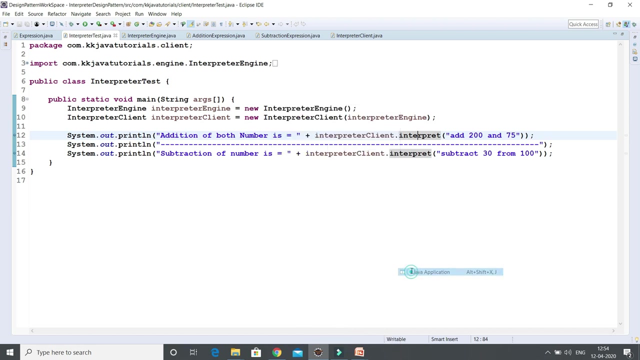 input data with the object of uh, addition expression or object of subtraction expression will be created. that depends on the our input right. if input content add literal, then addition expression will be called and input uh or data contains subtract endeavor some. i'm going to do three uh, let's say three hundred and let's say this is 40, then our grammar should be about two. 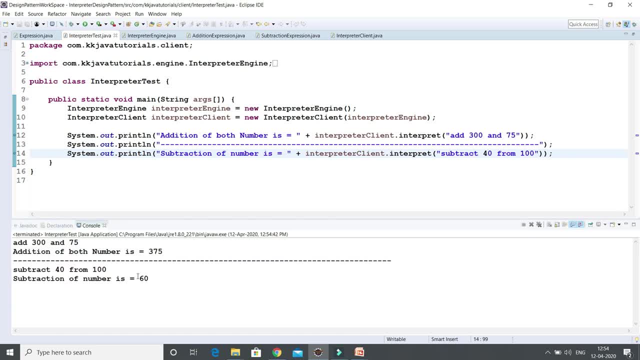 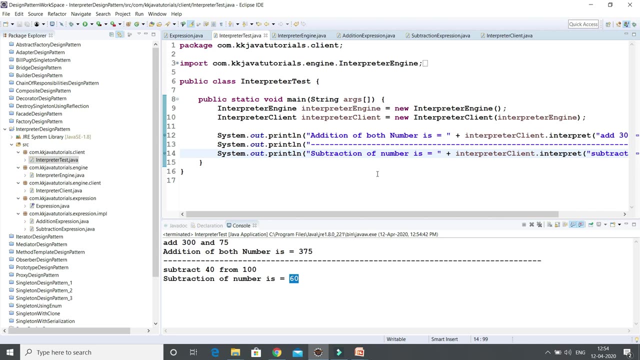 value of this expression as well, right? so here you can see now this is correct. sum, and this is the correct subtraction- is calculated by our grammar, right? so that's all i have in this video tutorial, guys. i hope you enjoy in this video. as far as source code concern, i will post this: 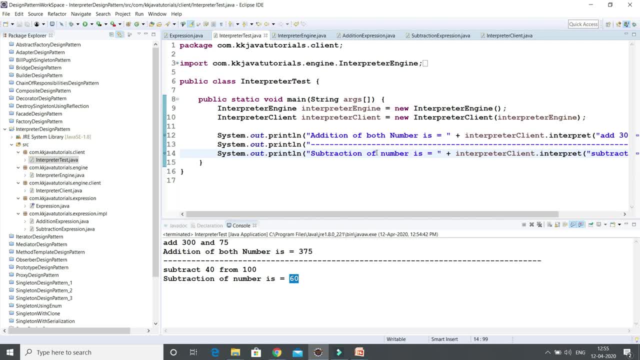 source code on my blog, akjavatutorialscom, and a link i will provide in the video description itself. so if you really like this video, then hit on the like button. if you did not subscribe my channel till yet, then please go ahead and subscribe kk java tutorials channel. guys, big thank you for watching this video. 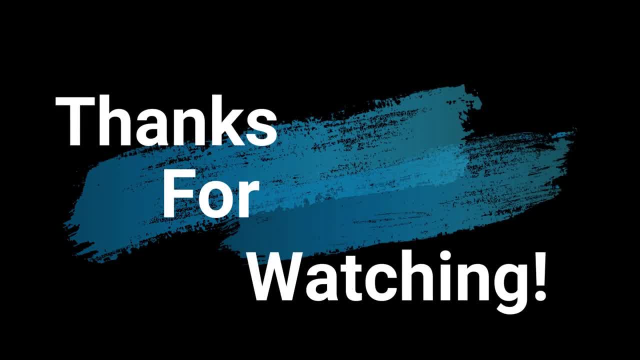 and see you there in the next video tutorial.